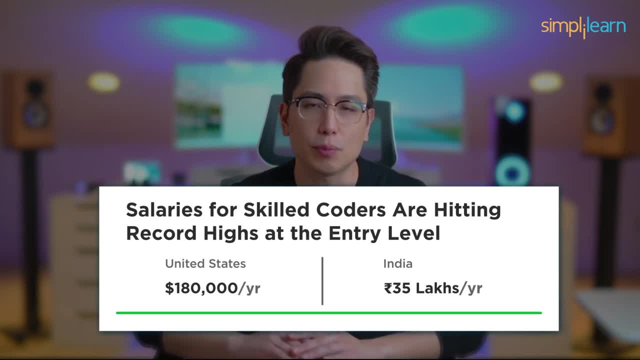 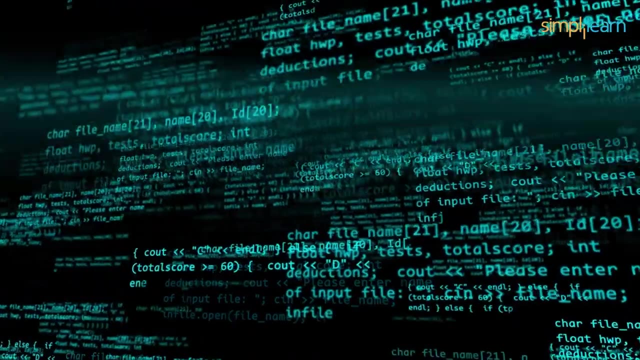 salaries for skilled coders are hitting record highs, with some professionals earning as high as $180,000 in US and 35 lakhs per annum LPA in India at entry level, promising a rewarding career. These languages aren't just code. They're shaping the future of technology, from AI to 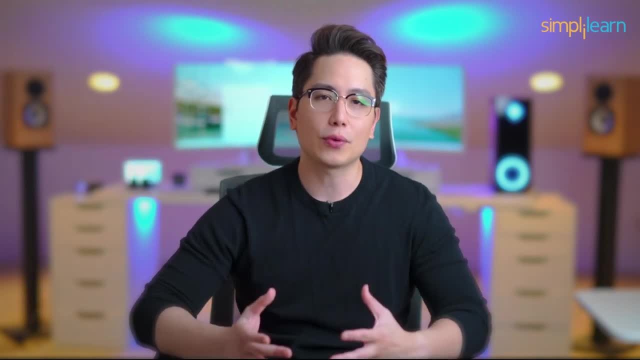 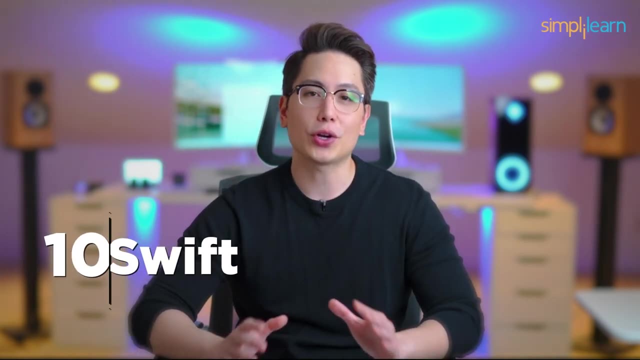 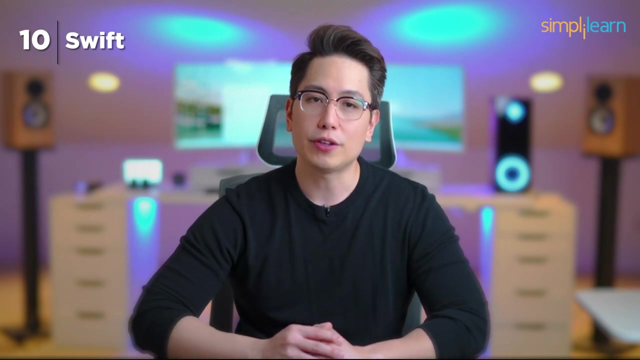 cybersecurity. Join us as we unveil the programming languages that are paving the way to innovation and prosperity. Number 10, Swift. Let's kick off with our countdown with Swift, the language that makes iOS app development a breeze. Swift, introduced by Apple in 2014,, is known for its exceptional speed and safety features. It's the driving force behind apps on your iPhone, ensuring that they run smoothly and efficiently. The demand for Swift developers is on the rise as mobile app usage continue to surge. Companies like Apple, Google, Uber and Airbnb are eager to hire Swift developers. 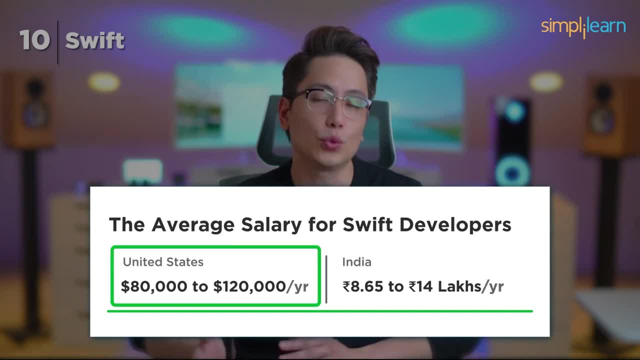 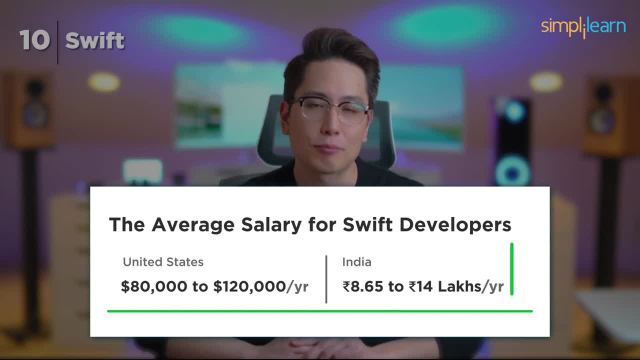 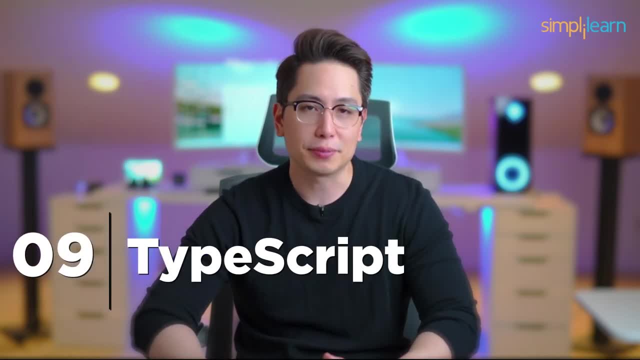 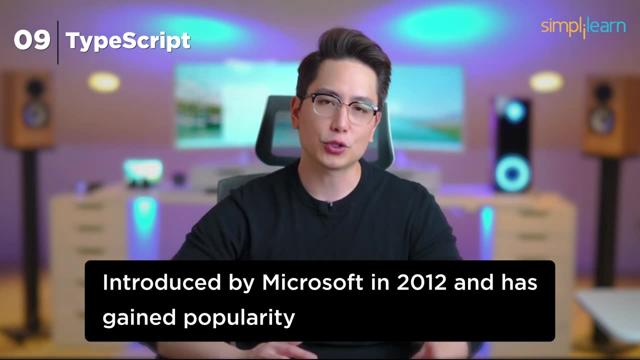 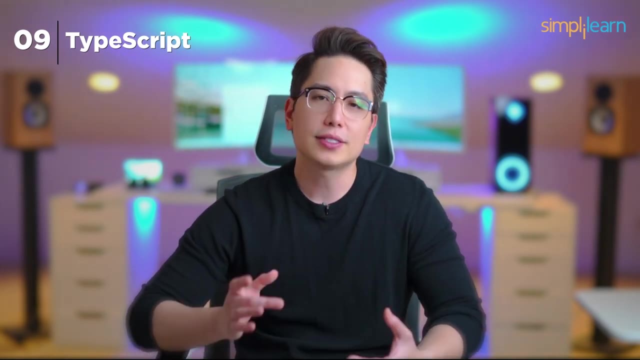 mobile app development. Number nine: TypeScript. At number nine, we have TypeScript, a superset of JavaScript. TypeScript was introduced by Microsoft in 2012 and has gained popularity for its ability to catch errors early in the development process. The static typing feature. 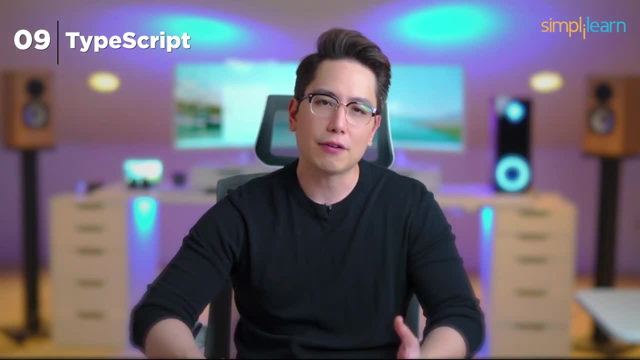 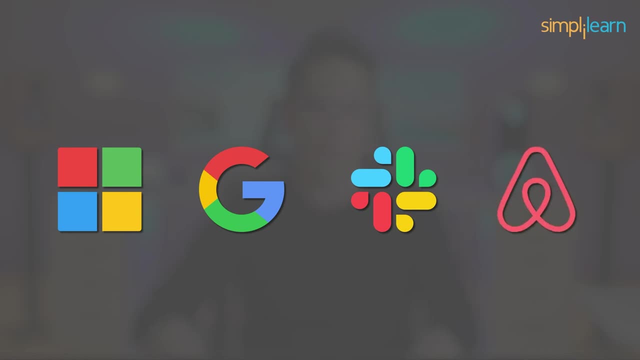 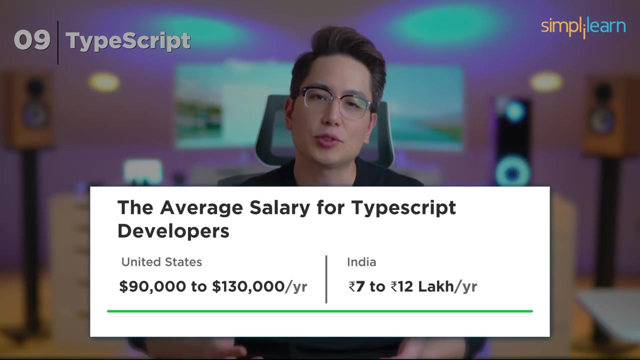 adds a layer of reliability to JavaScript, making it a favorite amongst developers. The type script is a popular tool for developers working on large-scale projects. Companies like Microsoft, Google, Slack and Airbnb recognize the value of TypeScript in building robust web applications. Skilled TypeScript developers can expect to earn between $90,000 and $130,000. 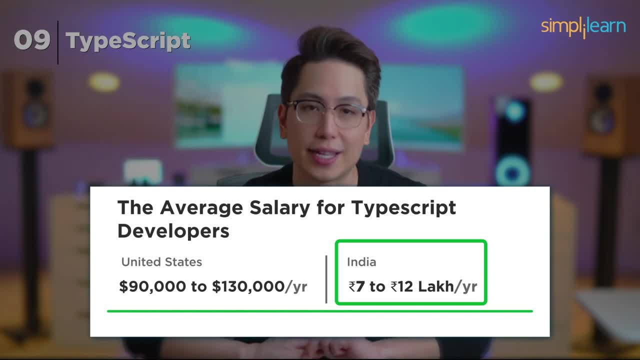 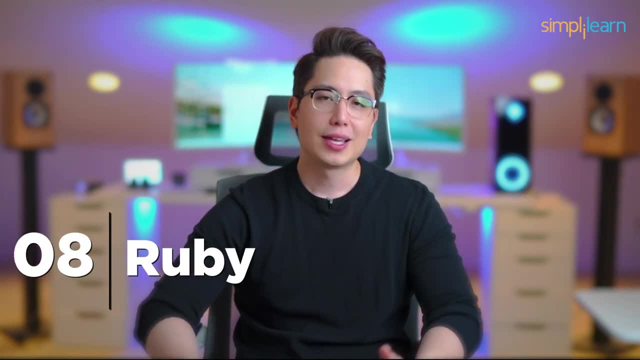 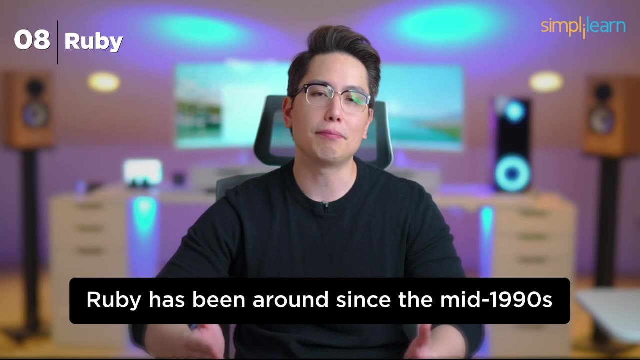 annually in the US and $7,000 to $12,000 lakh in India, making it a promising career choice for those seeking to master this language. Number eight: Ruby Claiming. the eighth spot is Ruby. Known for its elegant and developer-friendly syntax, Ruby has been around since the mid-1990s. and is the language behind the Ruby on Rails framework, which has revolutionized web development. Its simplicity and readability have made it a popular choice among developers. Companies like Airbnb, Shopify, GitHub and Basecamp appreciate Ruby's craftsmanship. Ruby developers typically earn salaries ranging from $70,000 to $120,000 a year. 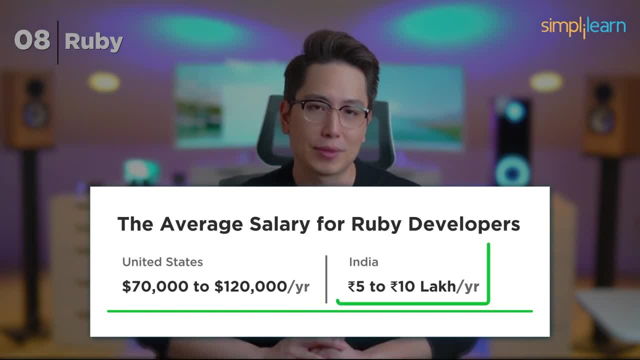 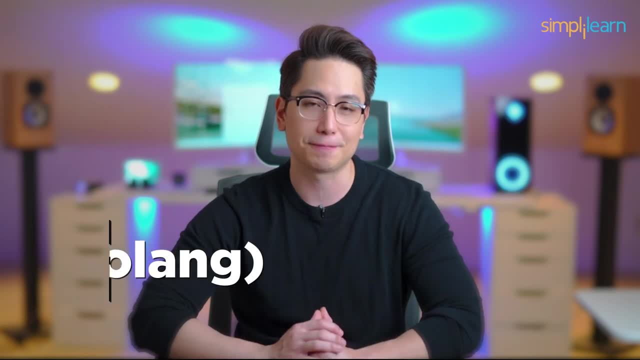 and $5,000 to $10,000 lakh in India. Its versatility in web development ensures it remains a solid choice for those looking to build web applications with ease. Number seven: Go Golang. Our seventh pick is Go, often referred to as Golang. 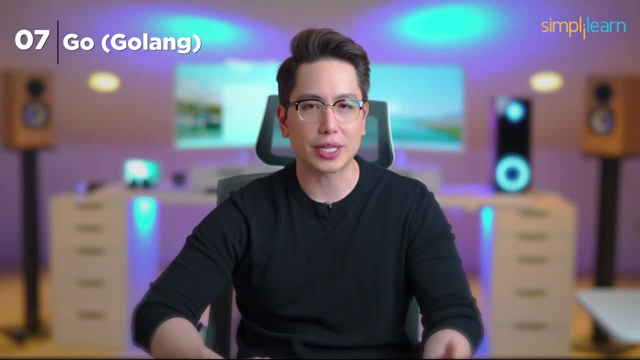 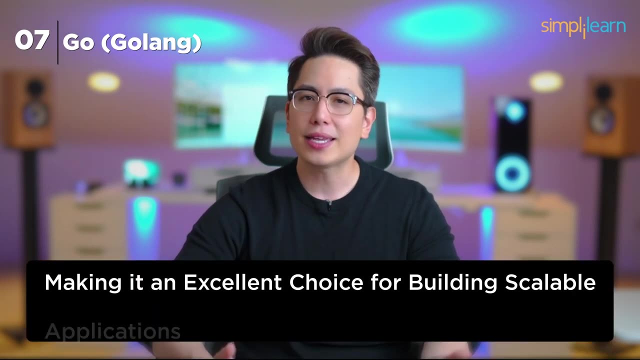 This relatively young language was created by Google in 2007 and is making waves in the development world. Go is celebrated for its efficiency and speed, making it an excellent choice for building web applications. Google is also known for its high-tech and high-tech. 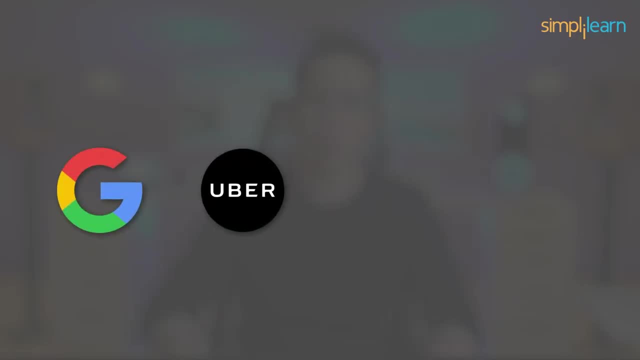 software and it's been around for a long time. It's been around for a long time and it's been around for a long time. It's been around for a long time and it's been around for a long time. Companies like Google, Uber, Dropbox and SoundCloud have adopted Go for various projects. 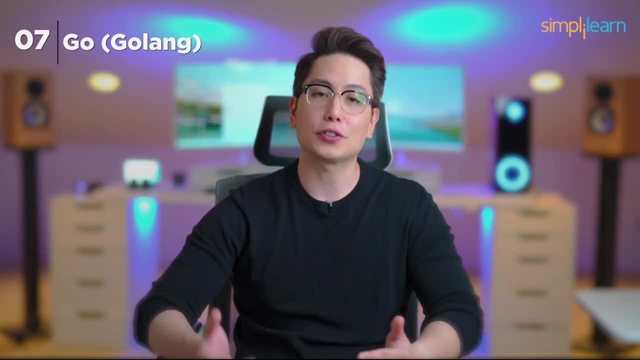 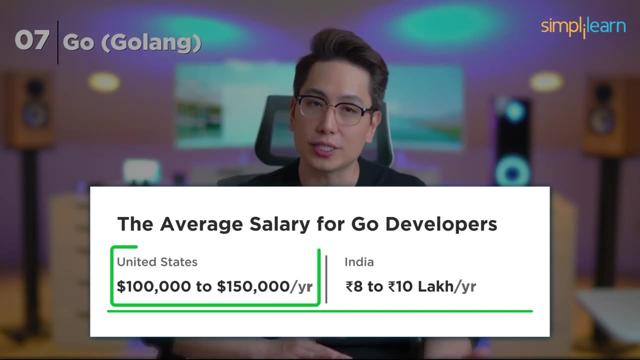 The demand for Go developers is steadily increasing and it offers a competitive salary range, typically between $100,000 and $150,000 per year in the US to $8-10 lakh in India, If you're looking to dive into the world of high-performance computing. 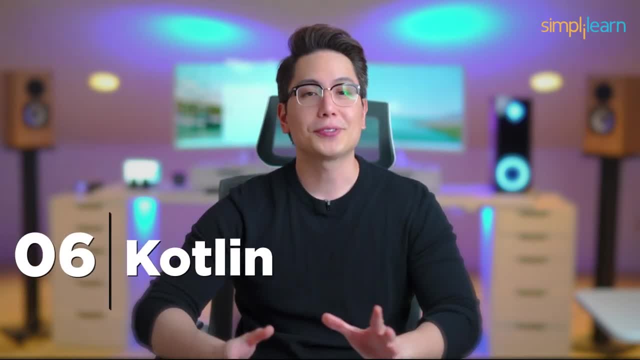 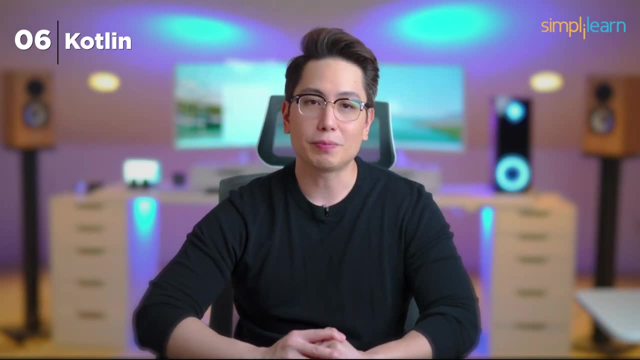 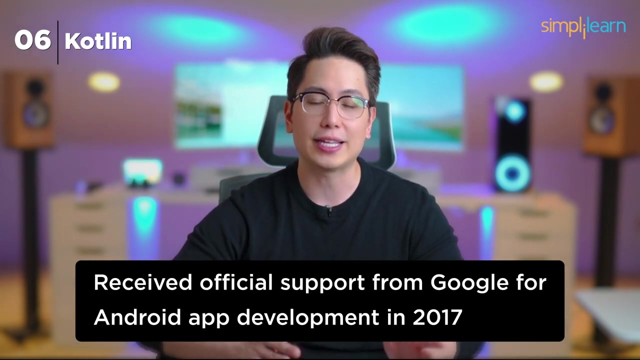 Go is a language to consider. Number six: Kotlin: Number six Kotlin- Landing at number six is Kotlin, the Android developer's best friend. Kotlin was introduced by JetBrains in 2011,, but gained prominence when it received official support from Google, from Android app development, in 2017.. It's recognized for its clean and concise code which reduces boilerplate and makes development more enjoyable. Kotlin has become the preferred language for Android app development in companies like Google, Pinterest, Trello and Basecamp are amongst its enthusiasts. Skilled Kotlin developers can expect to earn salaries in the range of 80,000 to $130,000. 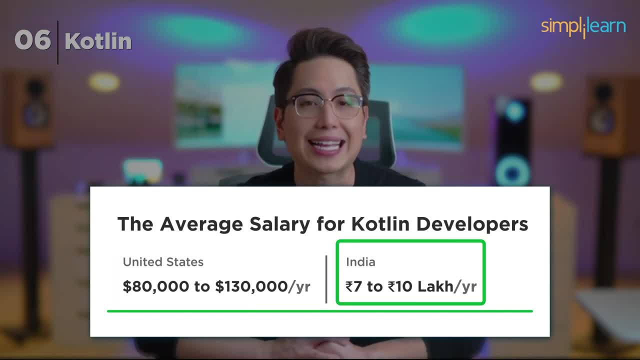 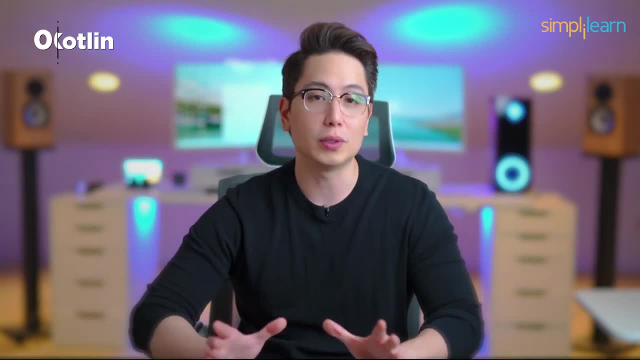 per year in the US to seven to 10 lakh in India. The continues growth of the Android app ecosystem, Kotlin, offers a promising future for mobile development. Number five: Python. Python takes the fifth position on our list. Created by Guido van Rosum in the late 1980s, Python has evolved into a new business, reflects a 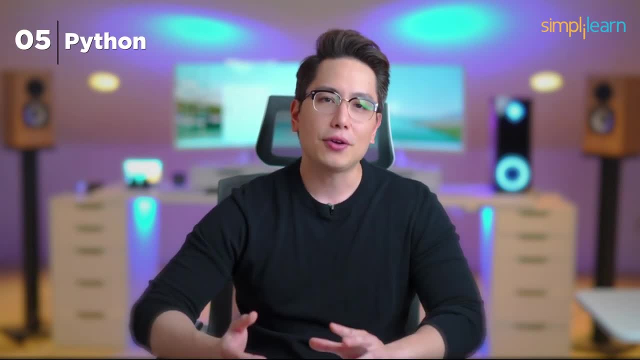 new goodness, Internet. Git has been goodness. Our natural 8 bin heavy atomic management has developed Google ads within preceding six decades. This is a cool studying experience. Number two Google. Number two Google: string fried app. Number two Google. 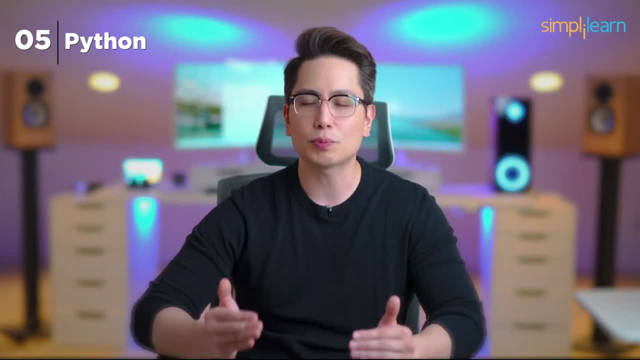 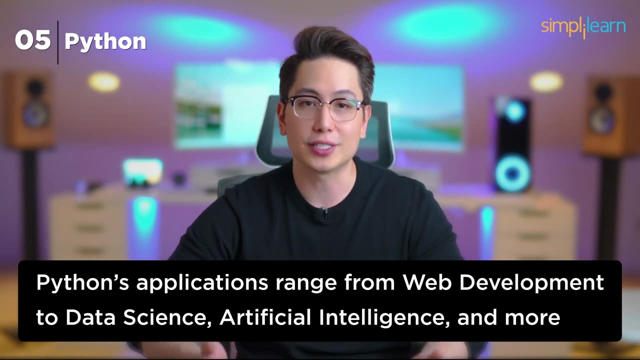 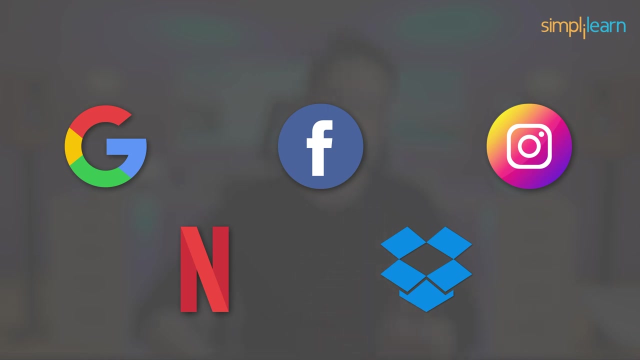 Google shares 10 cents a month próximo standoff, evolved into one of the most versatile and widely used programming languages. Python's applications range from web development to data science, artificial intelligence and more. Companies like Google, Facebook, Instagram, Netflix and Dropbox heavily rely on Python. 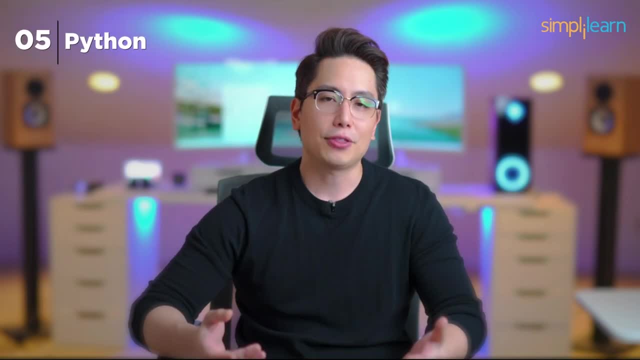 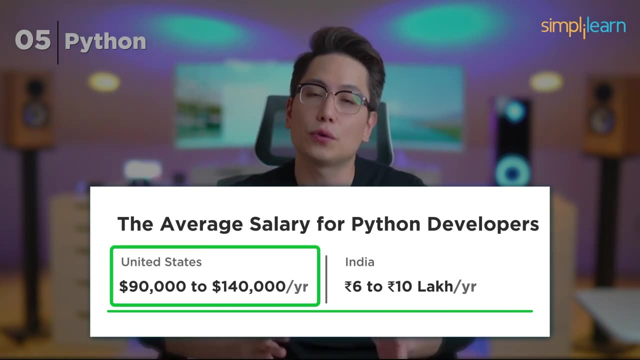 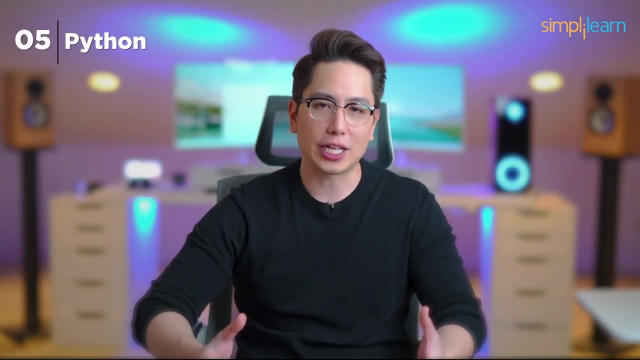 for various aspects of their operations. Python developers are in high demand and salaries for skilled professionals typically range from 90,000 to $140,000 per year in the US and six to 10 lakh in India. Its extensive library support and community make it an excellent choice. 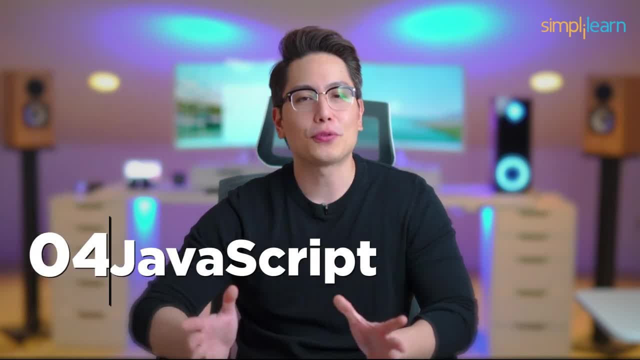 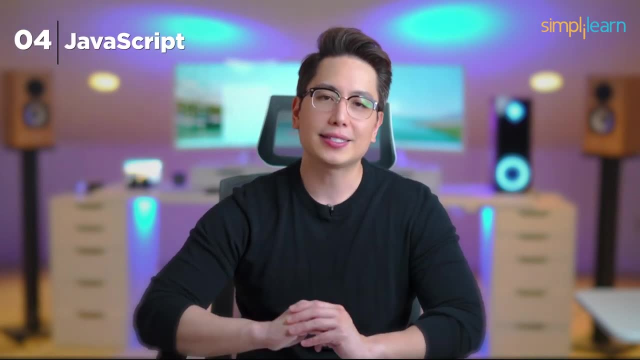 for those looking to dive into the world of programming. Number four: JavaScript. At number four we have JavaScript, the backbone of web development, Developed by Netscape in the mid 1990s. JavaScript has undergone significant transformations over the years. With the introduction of Nodejs, JavaScript expanded its reach to server-side scripting, making it a powerful and versatile language. Companies like Amazon, Netflix, PayPal and Airbnb depend on JavaScript to deliver interactive and dynamic web experiences. JavaScript developers typically earn salaries ranging from 80,000 to $140,000 a year in the US. 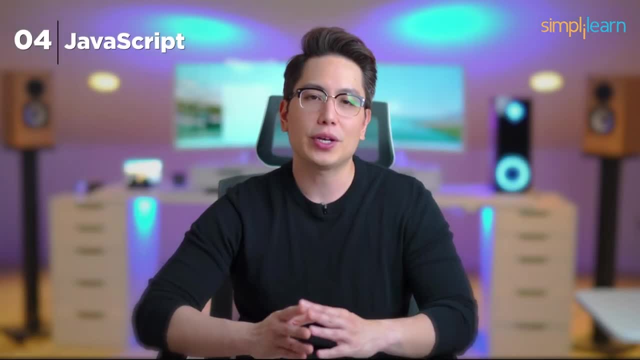 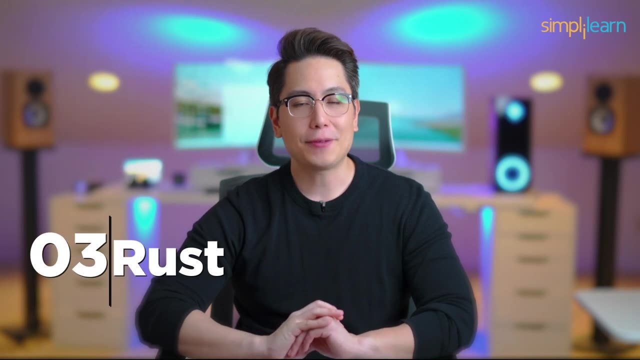 and seven to 12 lakh in India. Its ubiquity ensures that it remains a solid choice for every user, For any developer looking to excel in web development. Number three: Rust. Stepping into the top three is Rust, Known for its focus on safety and performance. Rust was first released by Mozilla in 2010 and has gained significant attention for its unique features. It's designed to prevent memory-related bugs and ensure safe concurrent programming. Companies like Mozilla, Dropbox, Microsoft and Red Hat have embraced Rust for various projects. 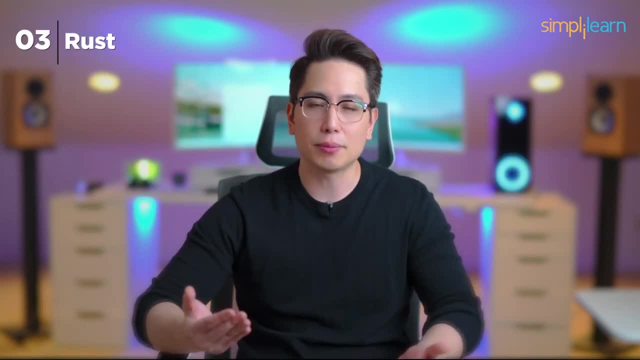 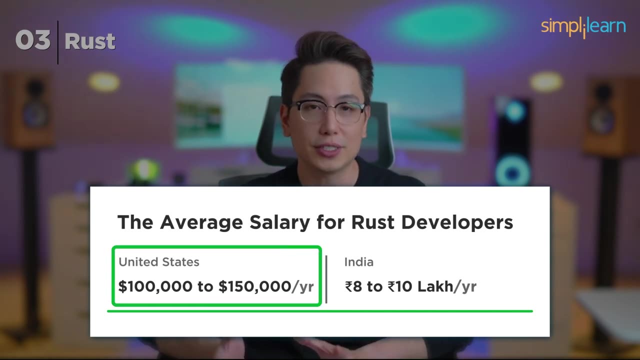 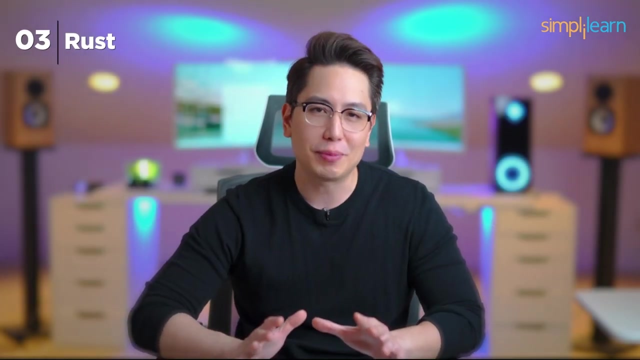 While Rust has a steeper learning curve compared to some other languages, the rewards for Rust developers are substantial. Salaries typically range from 100,000 to 150,000 per year in the US and eight to 10 lakh in India. If you are passionate about writing efficient 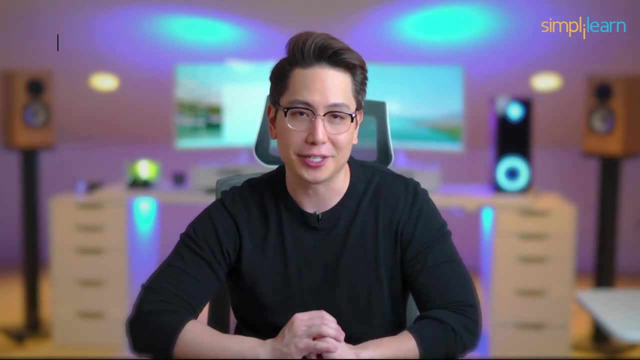 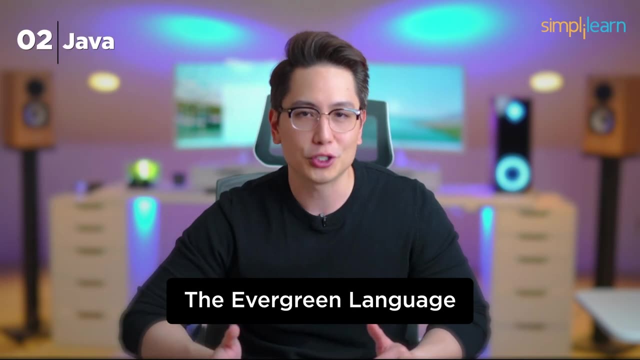 and secure code. Rust is a language worth mastering. Number two Java Claiming the second position is Java, the evergreen language. Java is the world's second-largest language developer. Java is the world's second-largest developer. Java was introduced by James Gosling. 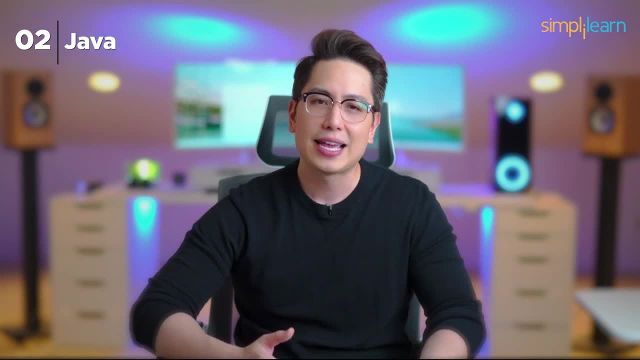 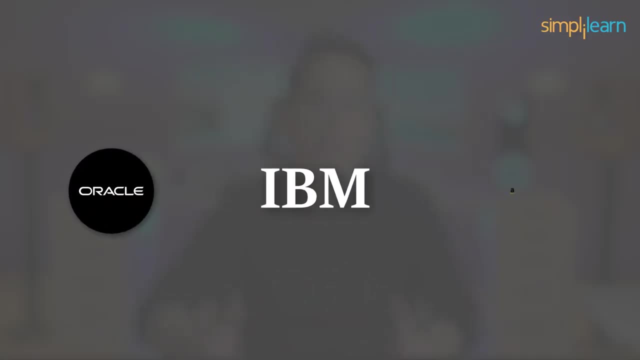 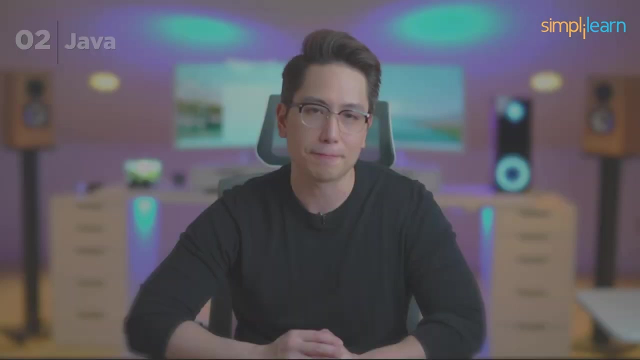 and his team at Sun Microsystems in the mid-1990s. It has since become the cornerstone of many enterprise-level applications. Companies like Oracle, IBM, Amazon and many financial institutions heavily rely on Java to keep their systems running smoothly. A career in Java promises job security. 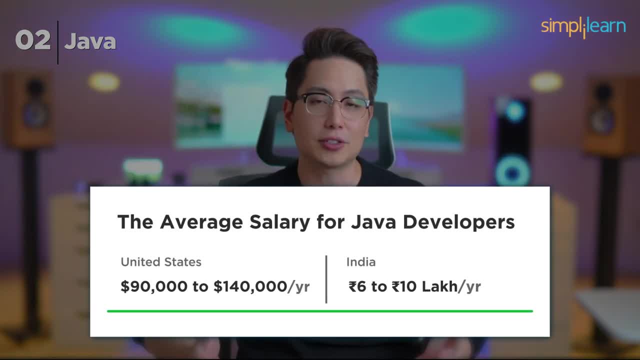